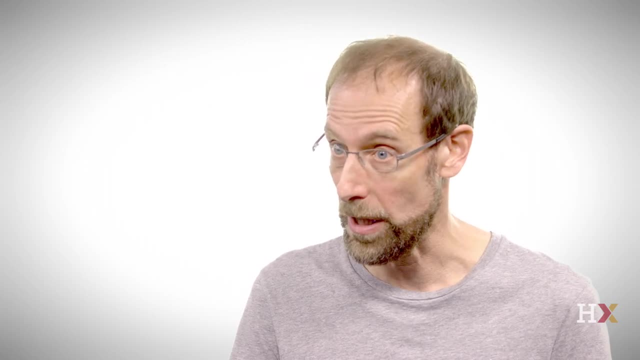 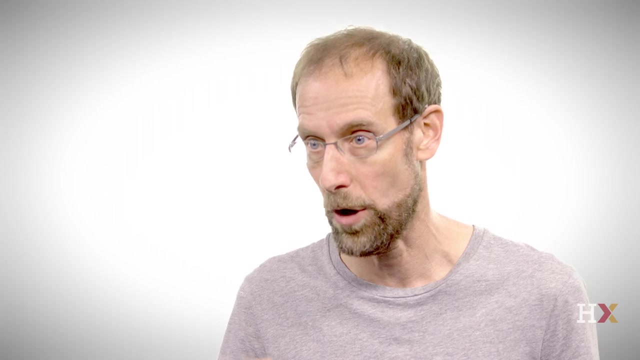 Of course there will be local scarcity of some fuels and there's a turbulence in the push and pull between oil and fossil fuels. But there are at least four forces that, in the long run, suggest that fossil fuels will be widely available. The first is technological change. The second is the geological diversity. 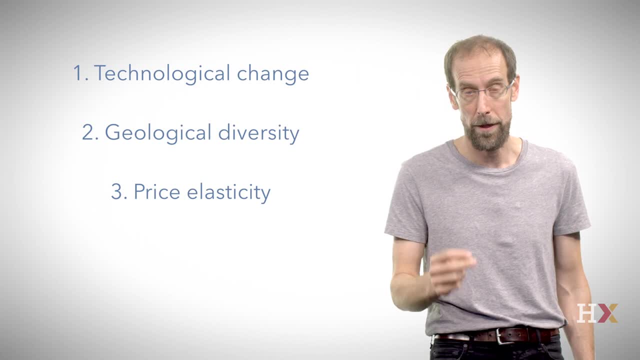 of the resource, The third is price elasticity And the fourth is interfuel substitution and conversion. In the next sections, we'll explore these four factors in order and look at how they explain the history of oil production in the world. First technological change: 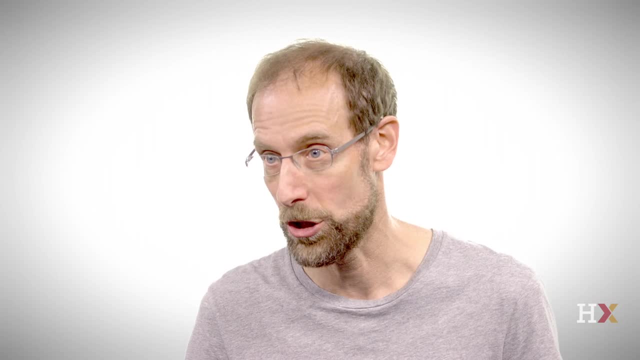 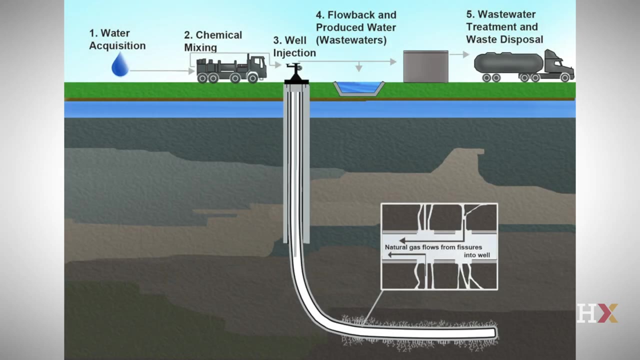 The technologies for finding and extracting oil and gas just keep getting better. Two examples: One is the shale gas revolution, where technologies for drilling long horizontal wells and for making fractures in precise locations that allow the oil or gas to seep out of rock that 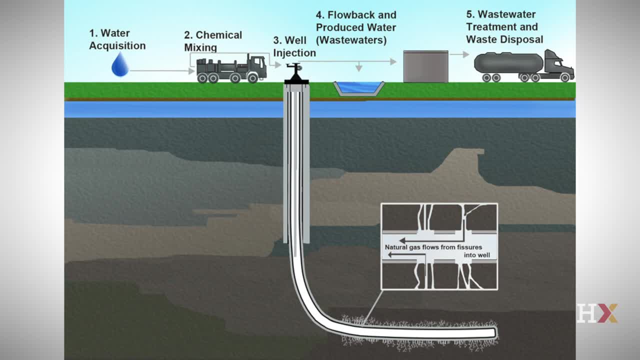 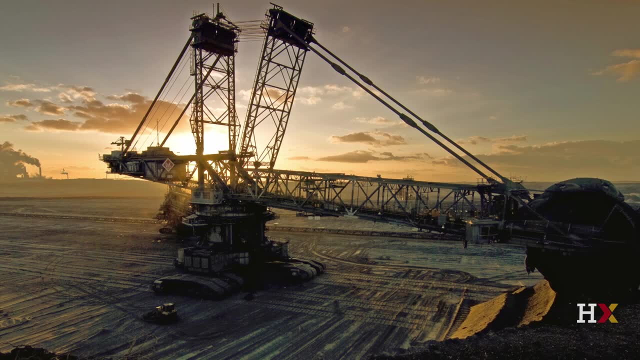 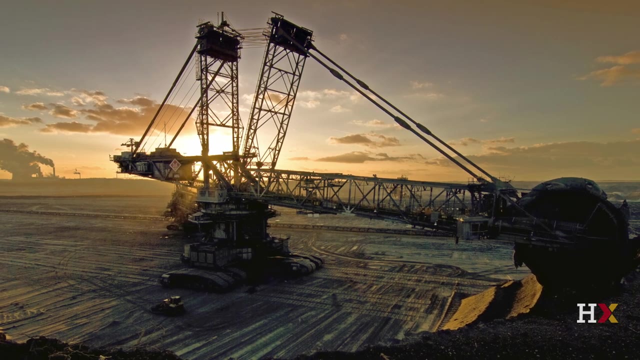 otherwise would be too tight, too impermeable to allow it to flow naturally- have allowed an enormous expansion of US oil and gas production using new technologies. Second, the gradual increase in the size and efficiency and now automation of mining equipment allows very large scale coal. 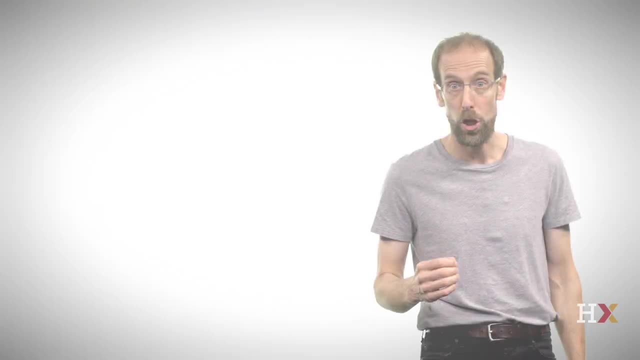 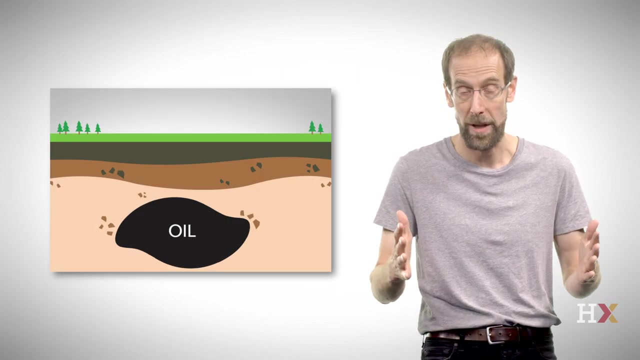 production at ever declining costs. Second, geological diversity. When one hears about an oil resource, it's very tempting to imagine a fixed reservoir like a tank And imagine that, as that tank is gradually depleted, you get to some point where it's all gone. 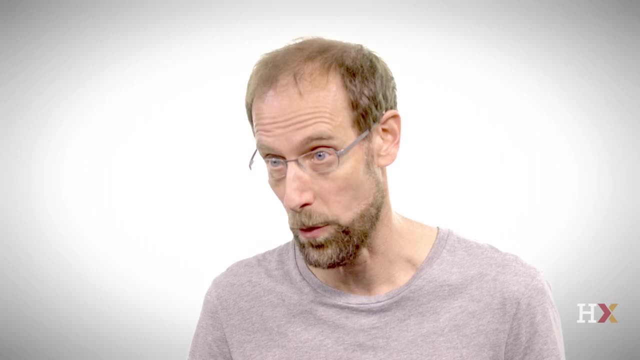 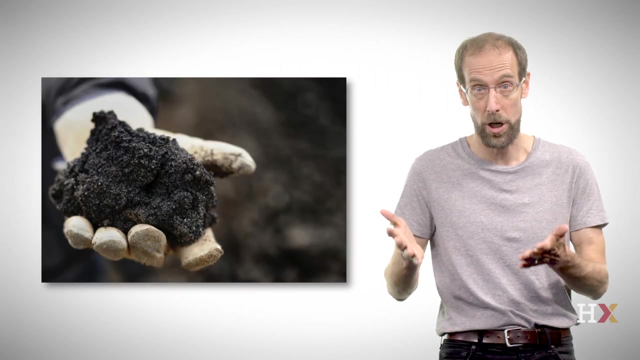 That's true for some conventional so-called volumetric oil reservoirs. Hydrocarbons occur in a vast diversity of forms. There are a. There are immense reservoirs, for example, of Canadian oil or tar sands. that are well-known deposits. It's easy to know precisely where they are, but they're very expensive to extract and 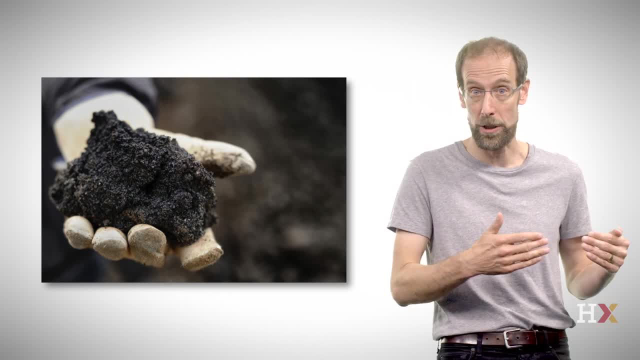 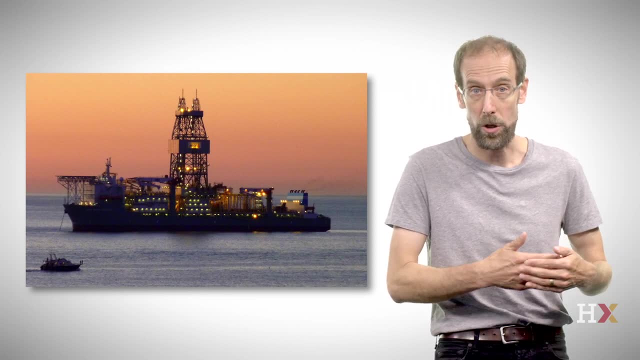 turn into oil. There are other deposits, like ultra-deep finds recently made off the coast of Brazil, where production is well understood, but finding them is very difficult. When you look across the whole world, there's enormous diversity of different kinds of oil. 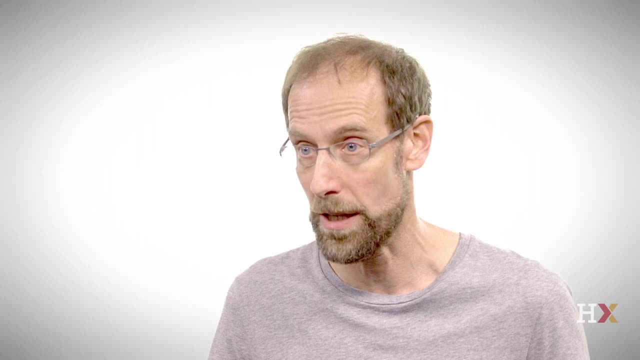 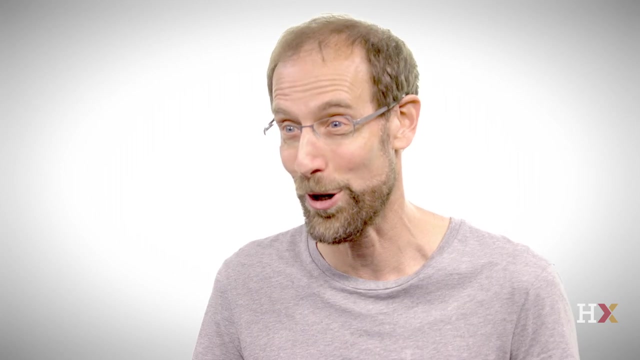 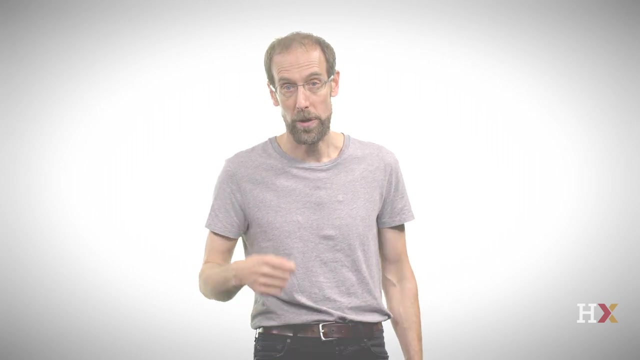 and gas reservoirs, And that diversity means that there's no reason to think about a single fixed supply. There are larger and larger supplies of materials that are harder and harder to get. at Third price elasticity: When prices go up, people work harder to get the oil. 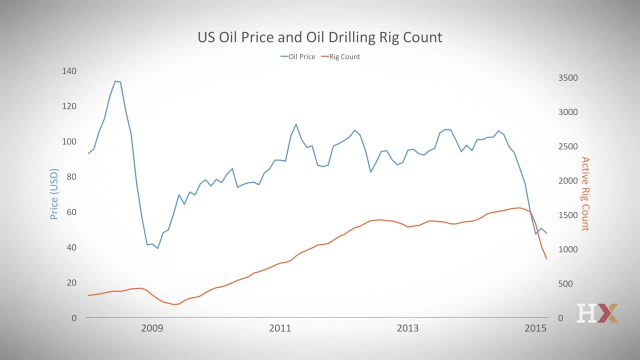 You can see this in this time series that shows the oil price along with the number of working US oil rigs. See how the two move together. They're correlated. Indeed, the technical definition of oil reserves is the amount of oil that can be produced using current technology at the current market. 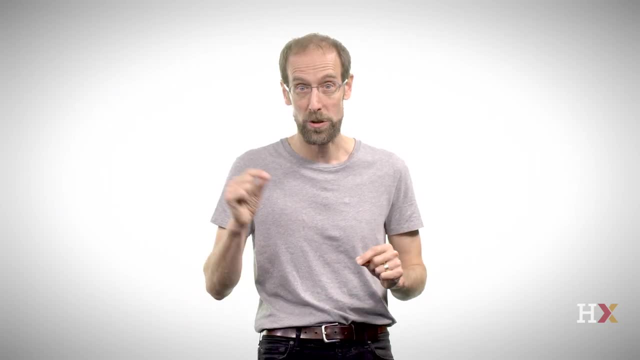 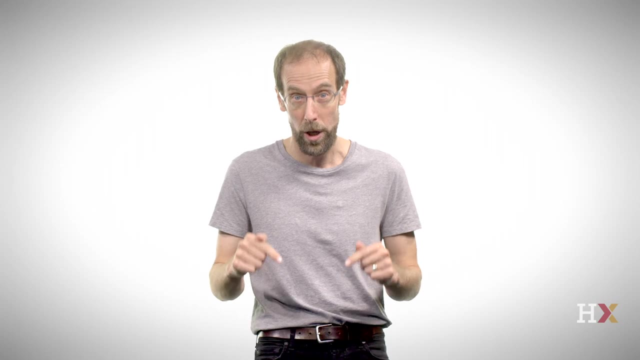 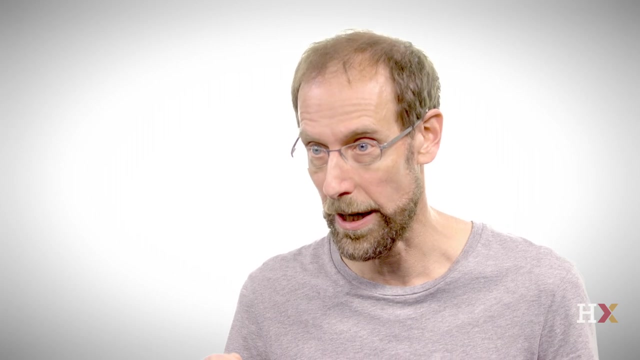 price. This means that if oil price suddenly goes up, oil reserves actually go up overnight with no change in technology and no change in the actual oil in the ground. Oil reserves are in this sense partly an economic definition. The McKelvie box provides a good way to think about the role of price, technology and geology. 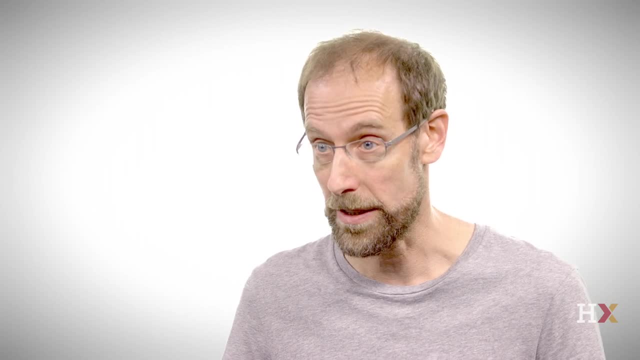 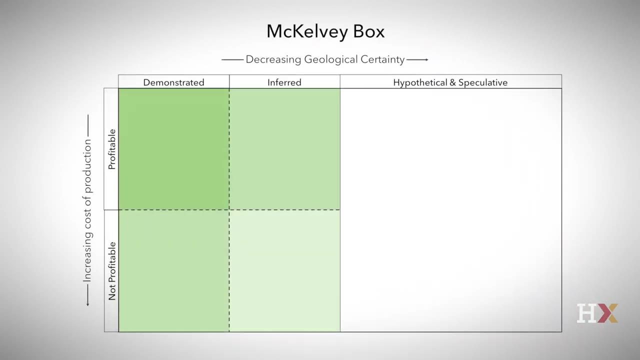 in determining the availability of a resource like oil and gas. This is a system that's used by economic geologists Studying both oil and gas and other resources like, say, minerals. The vertical axis shows the cost of producing the resource with current technology, while 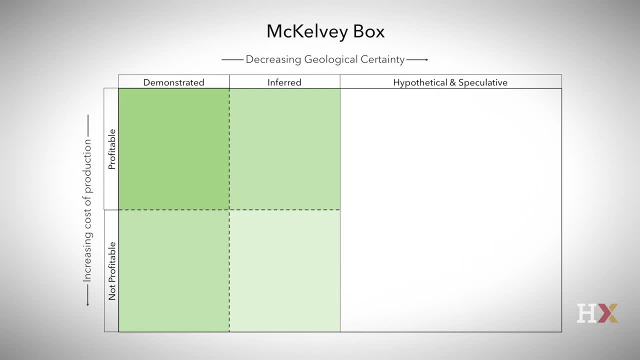 the horizontal axis shows the certainty that resource exists, geological certainty. So you can think about existing oil and gas reserves or resources on these two axes. The Canadian oil or tar sands, for example, are geologically certain in that we know precisely where they are. 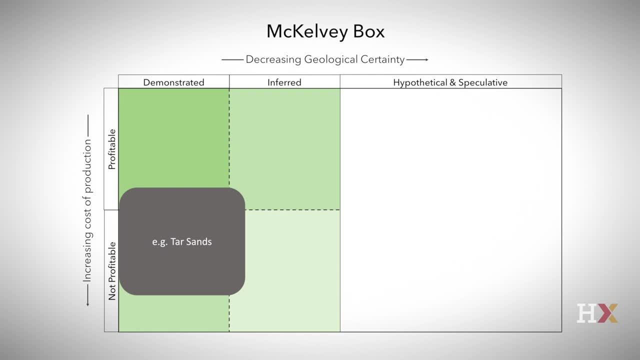 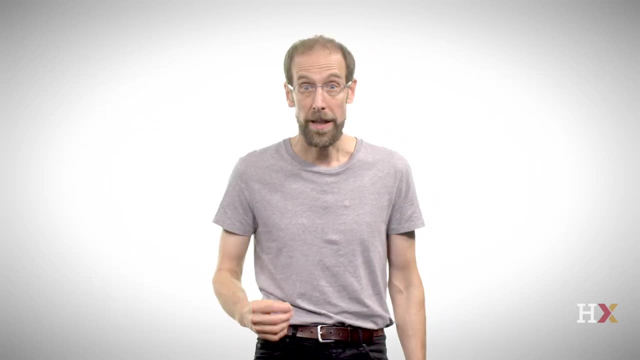 But the cost of accessing them, the cost of extracting that oil from the sands and turning it into a marketable product, has been very high, although it's gradually declining as the technology improves. Finally, the fourth factor driving the availability of fossil fuels is interfuel substitution. 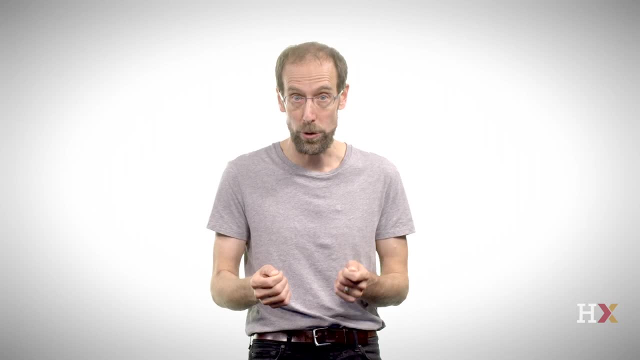 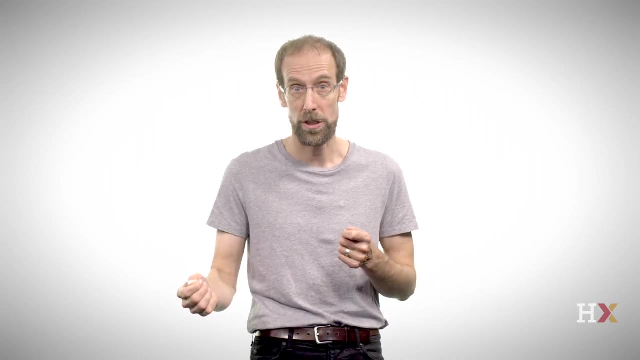 and conversion Substitution is when a user, for example an electricity plant, can choose between using gas or coal and oil, and so they shift to the cheapest fuel. This means that when one fuel is scarce, they can shift to another fuel, and this provides. 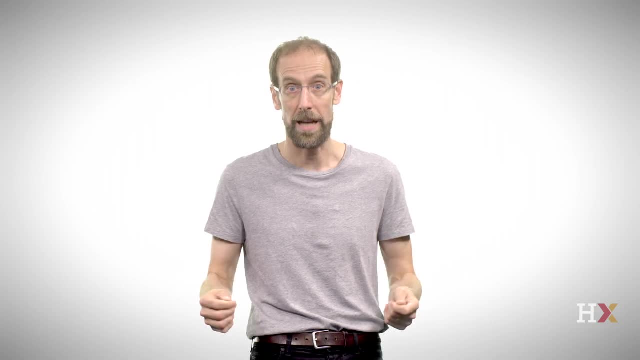 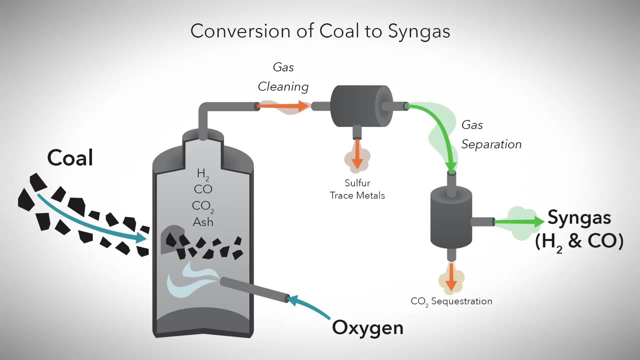 a kind of economic interchange between the three fuels, As well as an economic interchange when users actually switch. it's physically possible to turn one fuel into another. For example, we can turn coal into a gaseous fuel- so-called coal gasification- and we 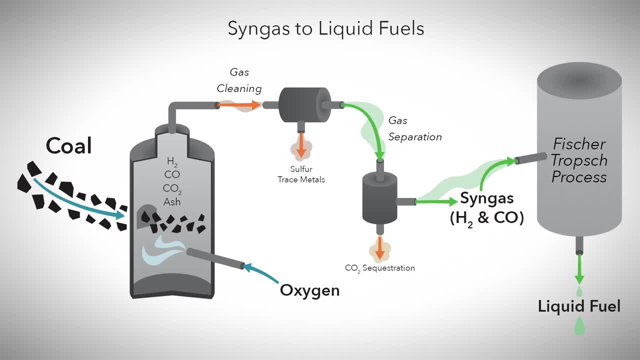 can turn gaseous fuels into liquid fuels, so-called gas to liquids. So in the world today, we both turn coal all the way into liquid fuels- much higher value fuels that are used for transportation- and we turn natural gas into liquid fuels. This conversion allows another kind of substitution, Separate from the economic substitution. it means that even if one fossil fuel runs short, for example that we run out of oil, running out of oil doesn't mean running out of hydrocarbon fuels produced from fossil fuels, because we could produce that same.